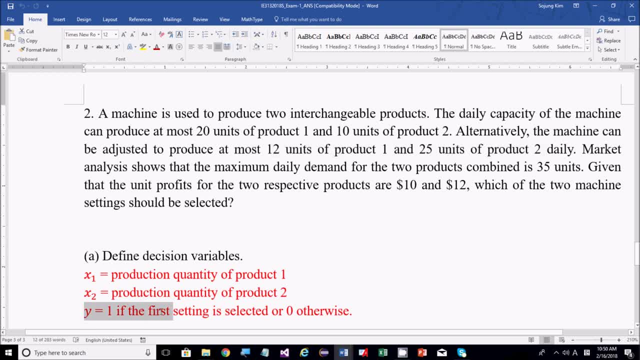 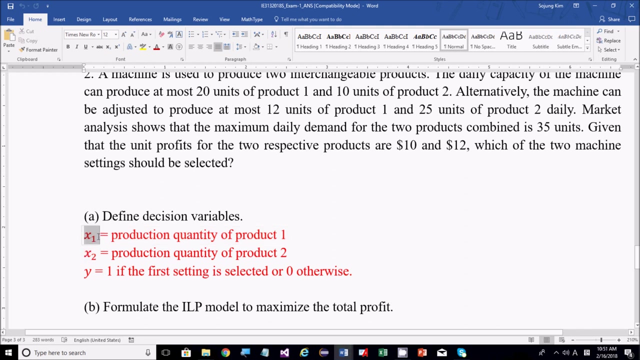 modeling. in my ILP model, integer program model, I have the Y binary binary decision variable, so it can be 1 if the first setting is selected. otherwise it can be 0, mm-hmm and also X1. I have two additional decision variables referring to production quality of product 1 and product 2, so 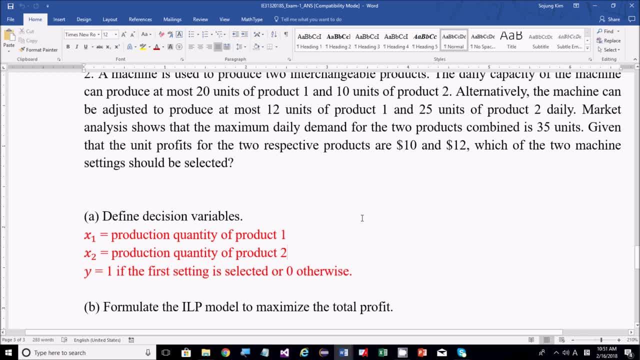 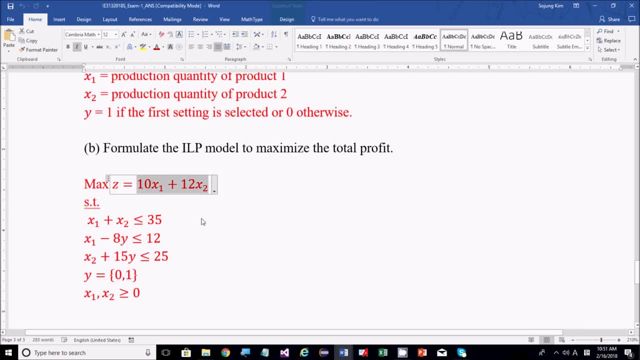 that we can calculate the total profit of the facility got it. so my object function only include two decision variables associated with production quantity of product 1 and product 2, because we know there is a decision value of product 1 and product 2. because we know there is a 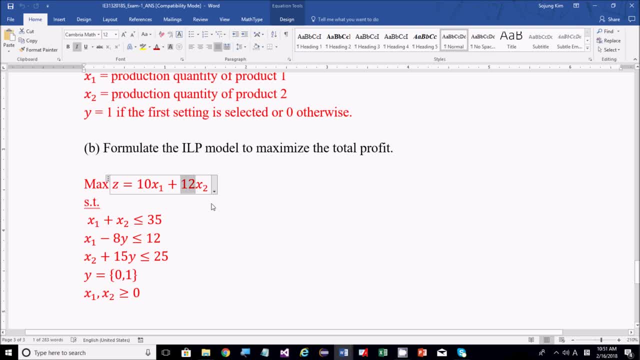 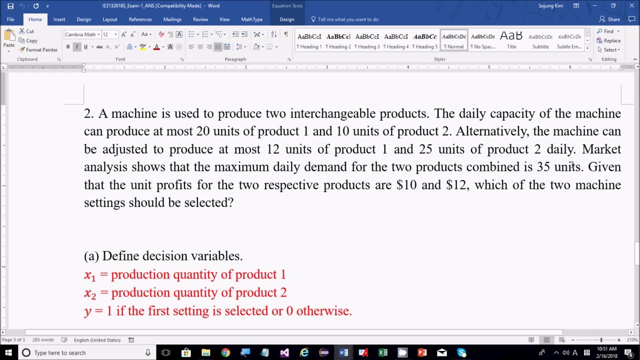 unit price, which is $10, and $10- $12, so you can make the your ILP model as a maximization problem. okay, including several constraint, got it? we know that total production quantity can be less than or equals to 35 because of this condition statement. right maximum daily demand for two products. 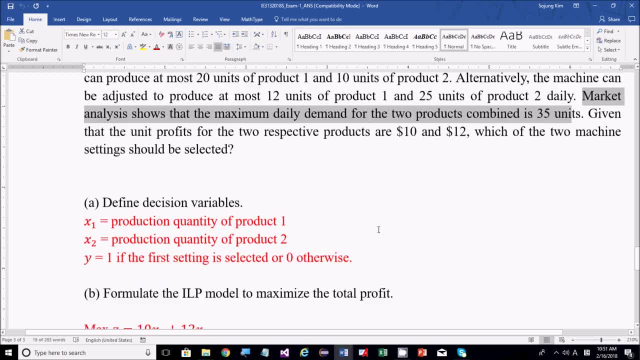 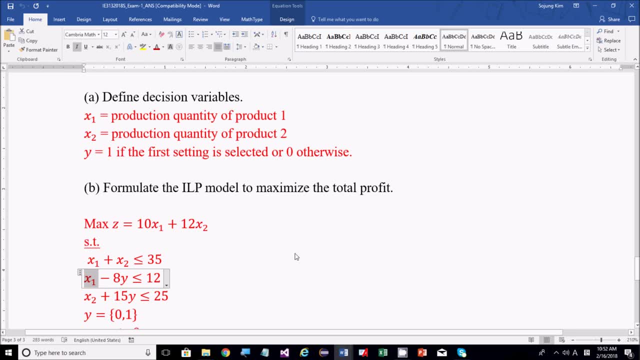 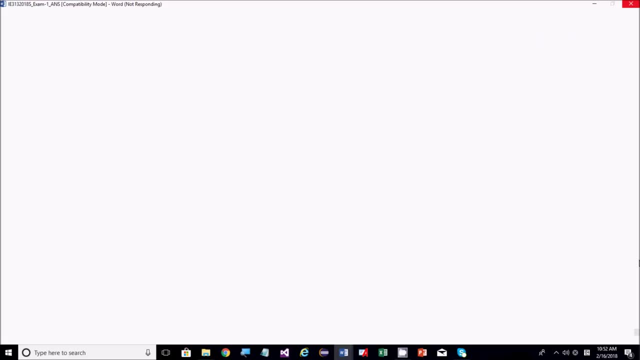 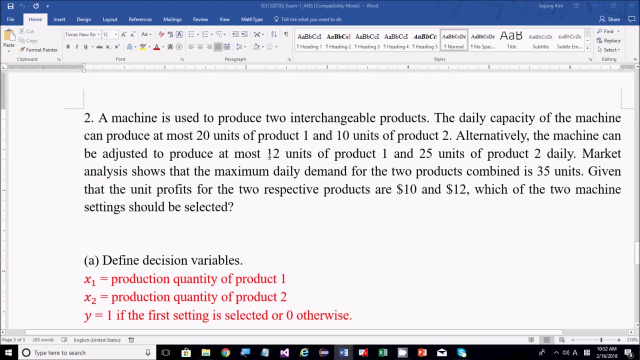 combined is 35 unit. so we have that one, okay, and then next one is very tricky. so initially, X1 cannot be greater than 12, especially when we select what, when you select which option, second option, mm-hmm. otherwise it can be up to a training unit, mm-hmm. so which means you should consider you. you have 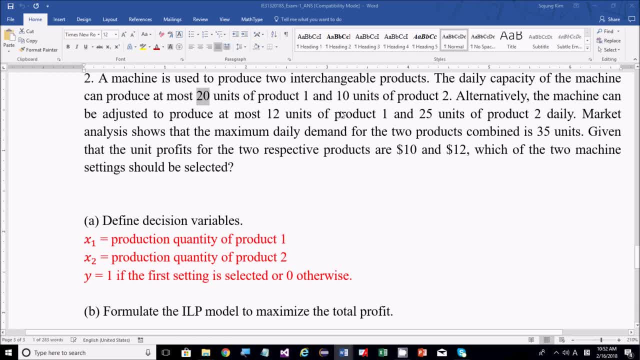 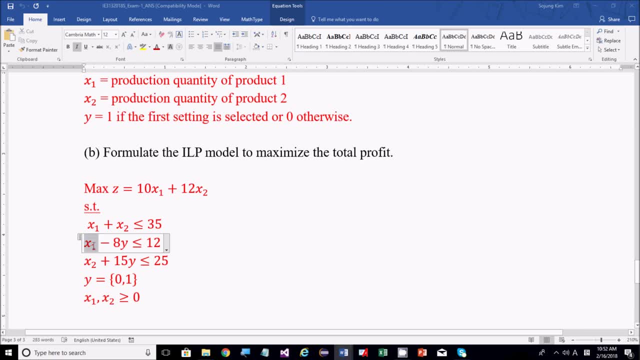 to combine these two requirements into the one constraint. associate the production quantity of product. 1 got it. so if Y value in my model, my value becomes 1, which means if we select the Y value becomes 1, which means if we select the function that is greater than 12 plus. 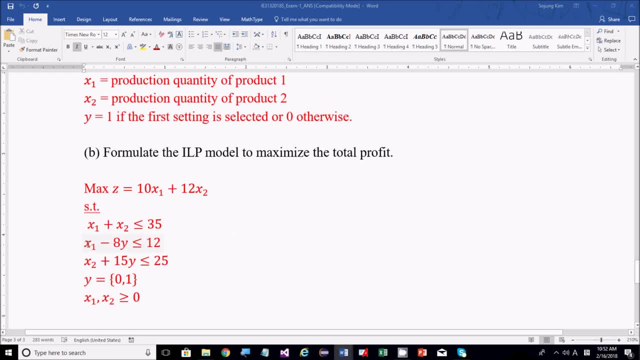 both the Y value becomes 0 and the product, quantity of product 1. now when we see that, count, gonna beavor how to make. haven't ever good at this test. okay, either way, you have to concentrate on sampling. choose the argument, limit short, down to say the definition rather. 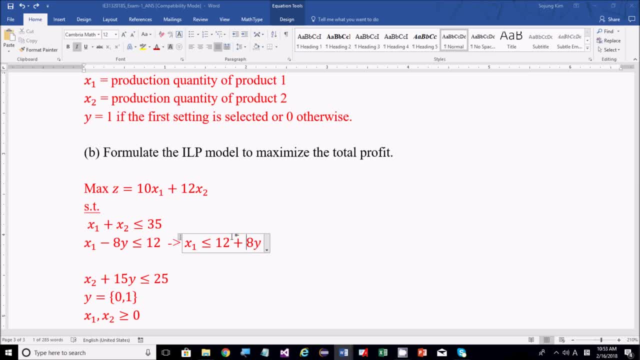 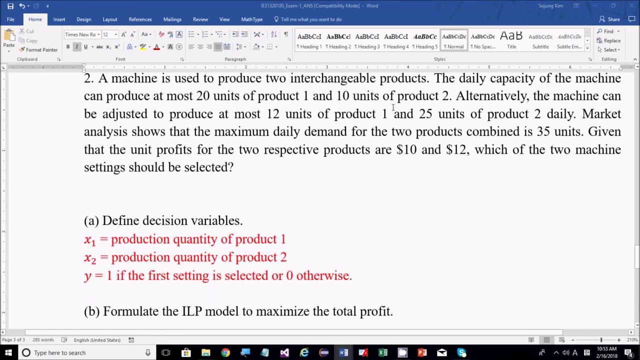 than order. so you could 그렇000. best do not be crazy. alright, now let's go pack. we select the second option. so this second constraint include eventually include two different requirements associated with the production quantity of product: one. similarly, you can add another constraint associated with the 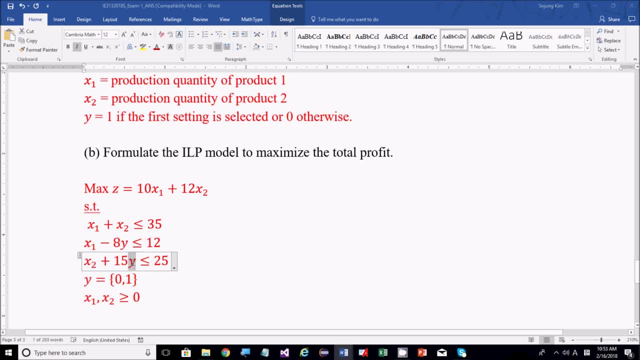 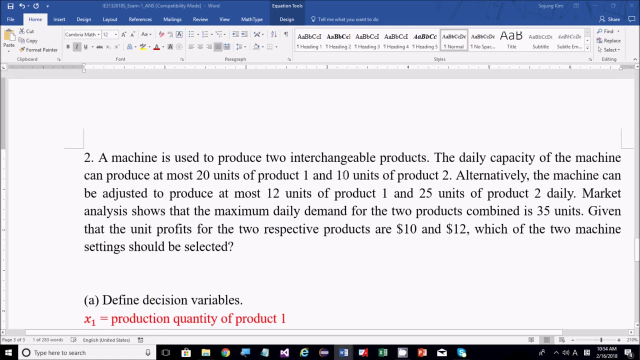 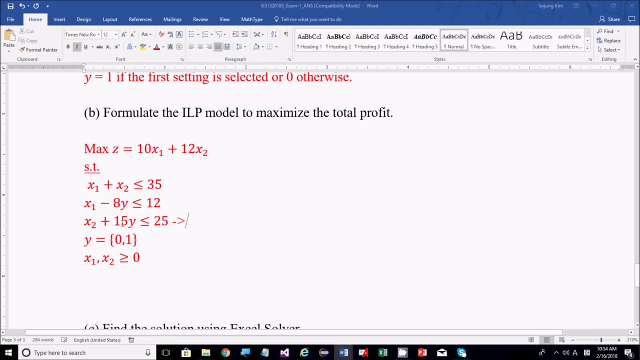 production quantity of product two involving Y variable. so in this case, if we choose the second option, the production quantity of product two cannot be greater than 25. got it? if we select the first option, then it becomes 10 unit. so eventually, if we select first option and then Y value, 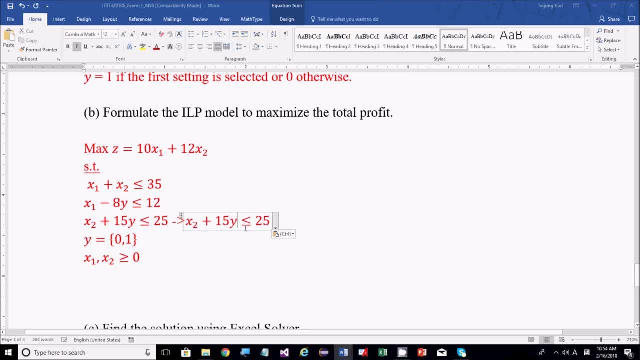 become one, so that our limit will be changed it to 10. mm-hmm got it. when y1 is 1, in other words, first option is selected. and also we know that y is a binary variable and x1, x2 is, a is greater than equal to 0. 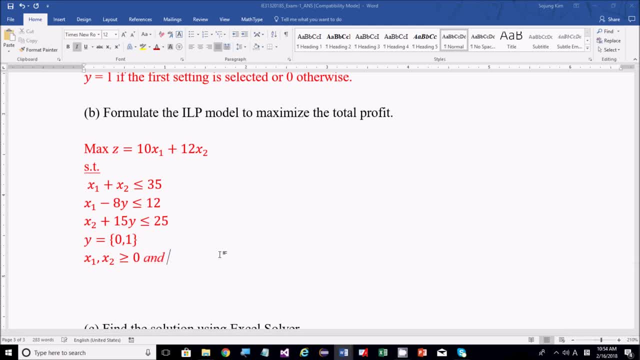 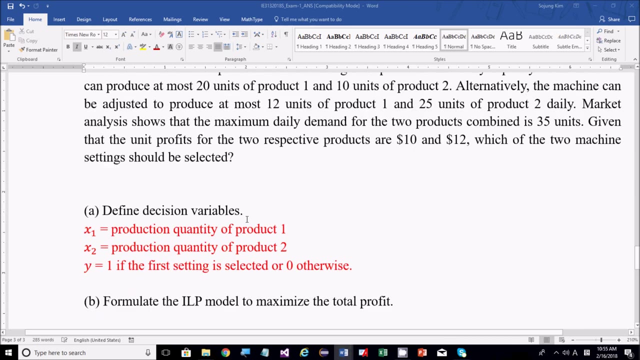 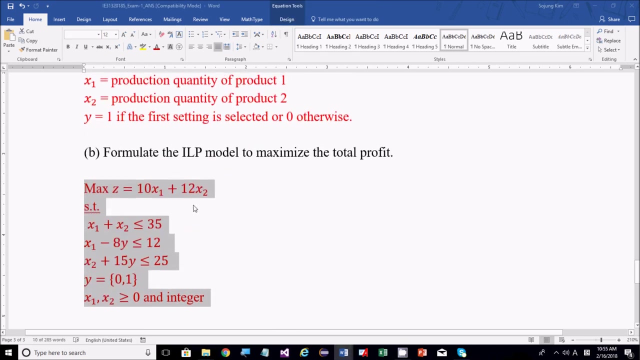 and they are an integer mm-hmm. so here our ILP model should be like this. otherwise, if you decide to use two different, like a Y variable for the selection of each option, you should, let's say, you have one y1 and then if you have y2, 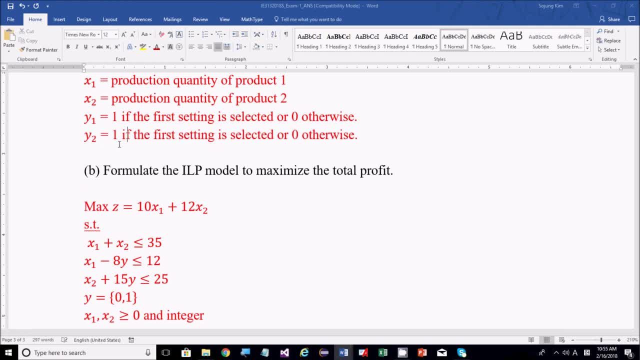 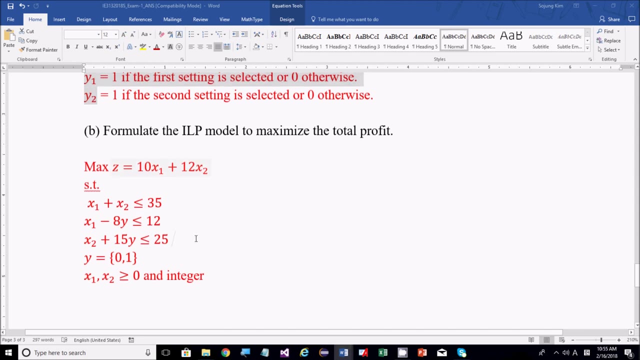 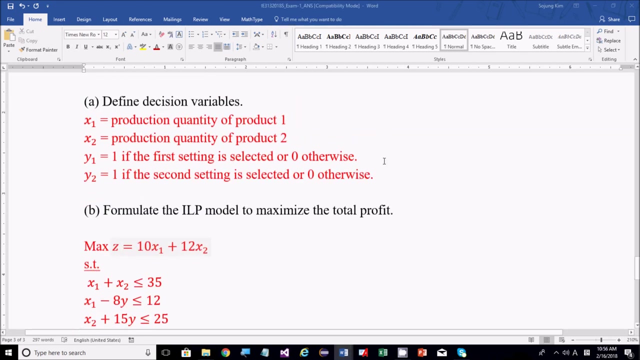 alternatively, if second oops setting selected, then you have to add one more constraint, which is which show the relationship between what y1 and plus y2 must be one, so that you can only select the one of the option. got it okay, so let me go back to the my original model. 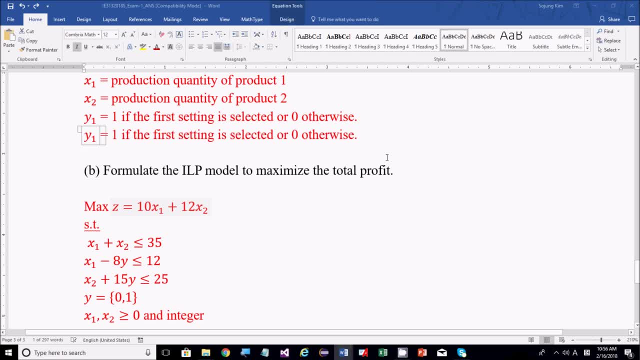 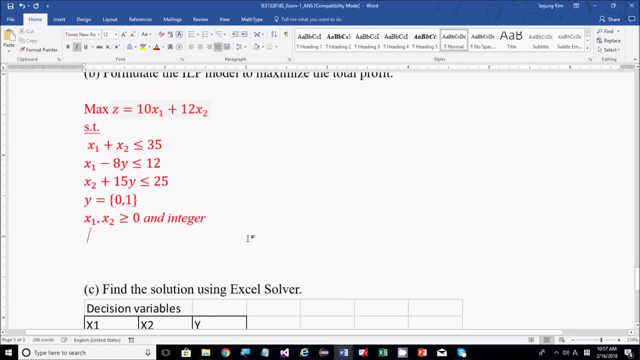 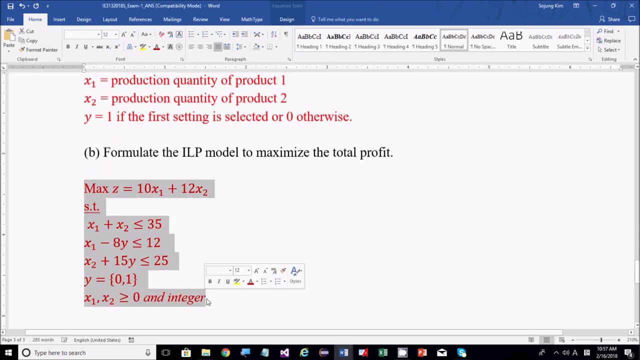 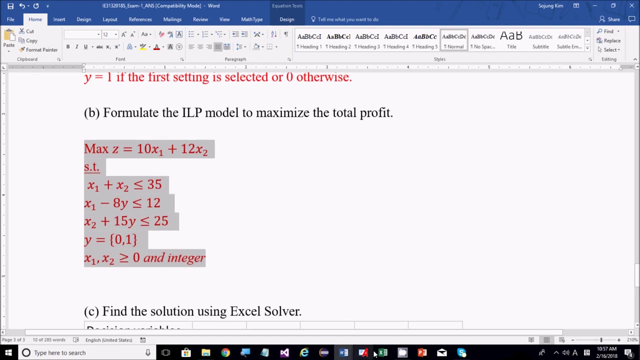 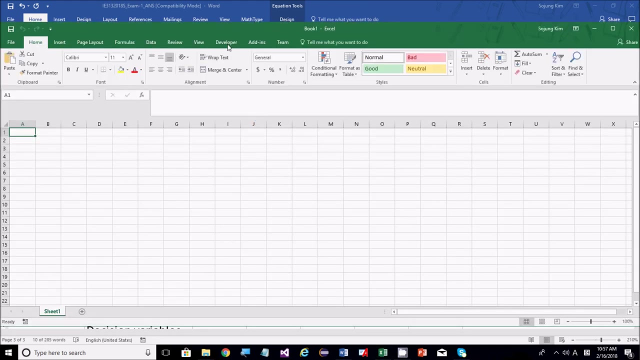 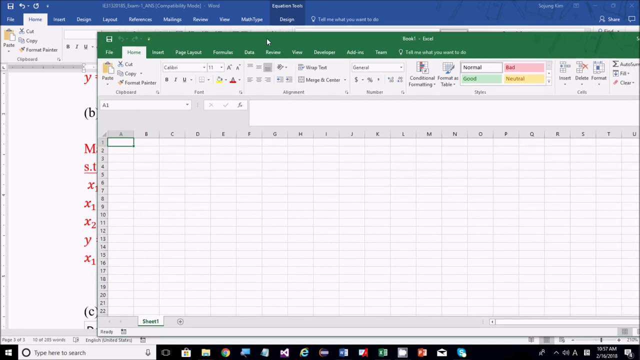 so let's solve this model using solver, so eventually we will get the solution. but let me let's use the Excel directly to get the solution, ok, ok, ok, ok, ok, it takes time to open the problem program in my computer anyway, so in here, just checked whether you are. you should check whether you. 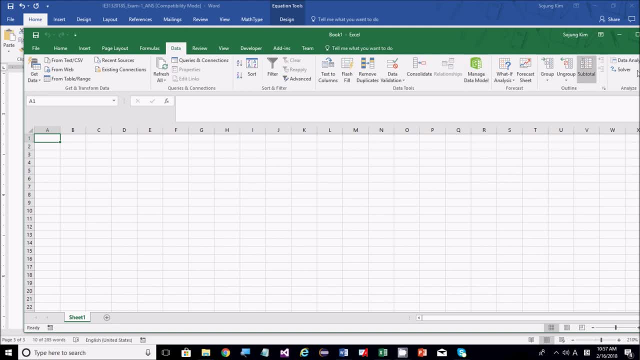 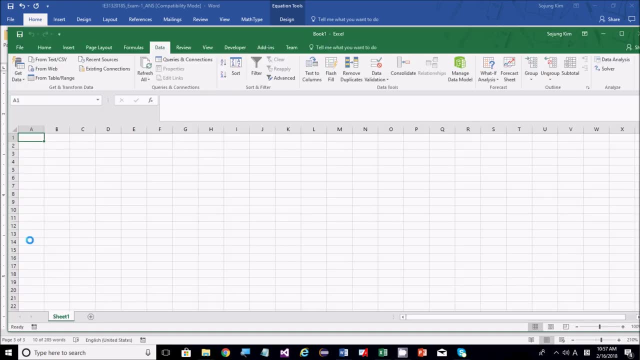 have the solver in your Excel or not. if you don't have the solver here, and definitely you can go to the option and then click the add in so that you can add solver, adding into your Excel. but my case, I already have one. I already did this. 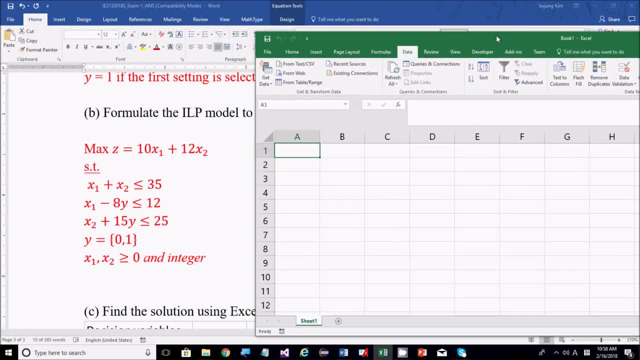 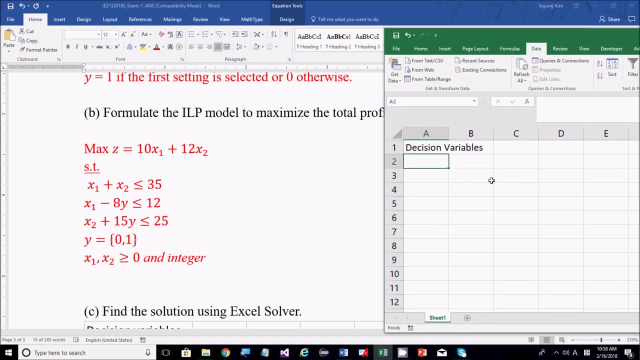 first of all, whenever you use, whenever you use the Excel, yes, you have to define the decision variable. first we have two decision variables and then we have about one right last one is binary variable and then we have multiple constraint relate to these three variables and then we have multiple constraint- wait to do three variables. 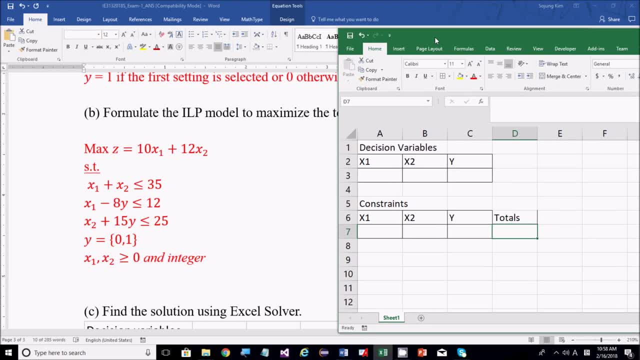 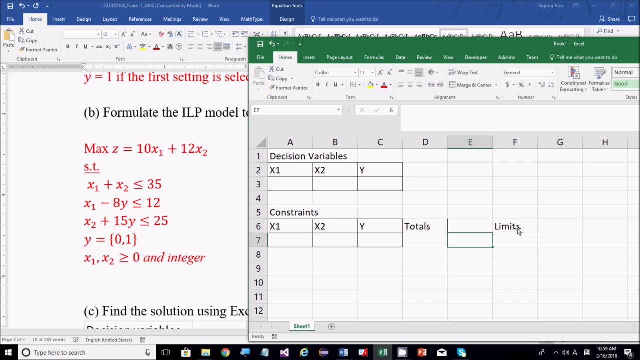 so we have to calculate the left hand side of each constraint and its right hand side, so inequality will be less than equal to for three options, that's three constraints, right, okay? so what's the coefficient of the x1 in the first constraint? so 1, 1, and this is 0. 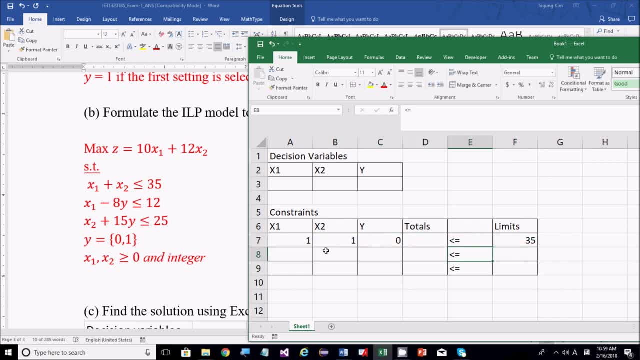 because there is no y in the first constraint and the limit is 35. same thing. next one is 1 and there is no x2 in the second one here. so it is minus 8 true, and limit will be 12. last one is 25, third one, and then there is no x1 in the third constraint and x2 equals to 1. 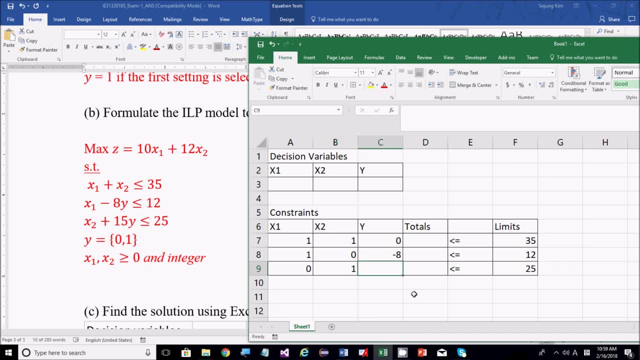 I mean the coefficient of x2 is 1 and 15 here, which is a constraint of the y, mm-hmm and total. you can use some product function including the three decision variables and their coefficient, and their coefficient so that you can calculate the value of the left-hand side in Excel and press f4 so that you. 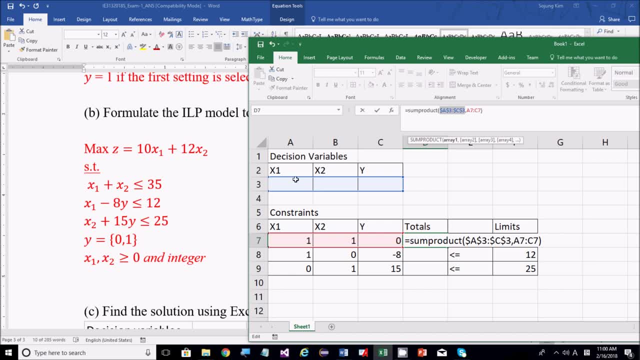 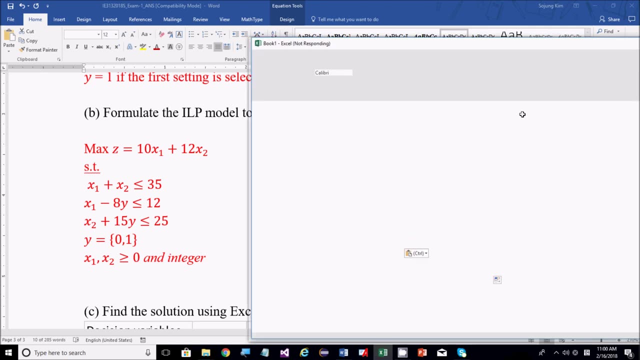 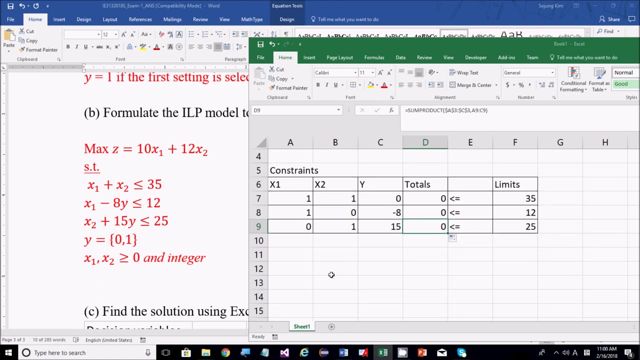 can use our absolute reference function, which is the value of the x1 in the first constraint and the limit will be less than equal to x1 in the second constraint and x2 equals to 1, which will reference the d3 decision variable. okay, and then you can just use the autofill function. and last one is objective. 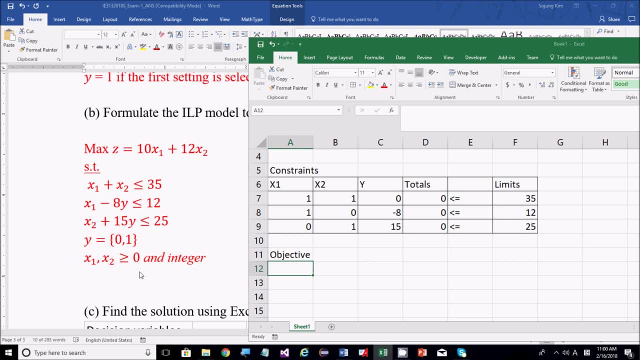 you don't really need to care about these two constraints, because we can put these constraints in solver directly. object function is the same thing: x1, x2, y, and the coefficient of the x1 is 10, right here, so 12, and this is 0, and still you can just copy and paste some product.